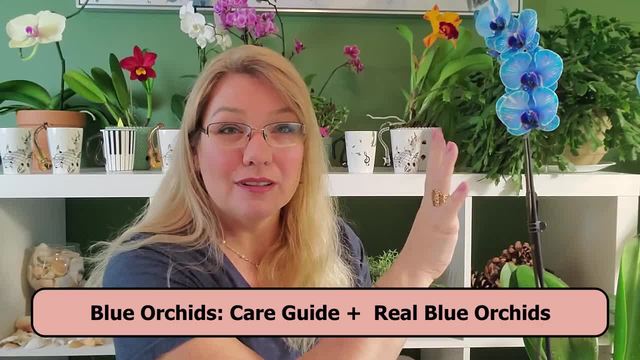 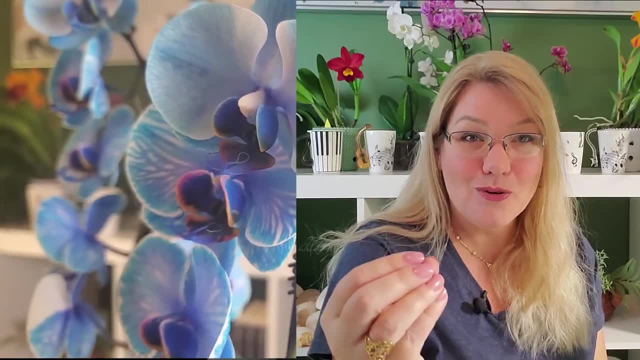 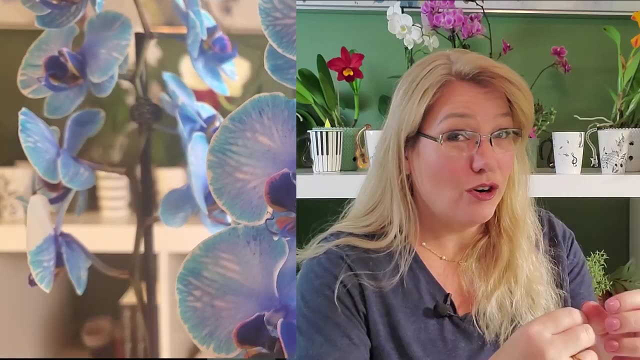 So in this video you're going to learn how to care for this beautiful blue orchid, and I am going to mention four real blue orchids that can be found in nature where man has not manipulated and has not genetically induced a darker indigo color. So I went to the supermarket this morning and I bought. 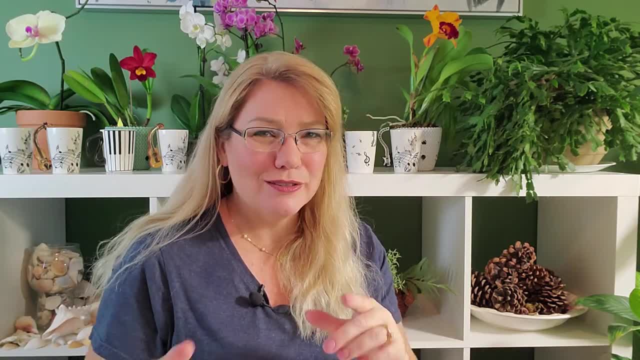 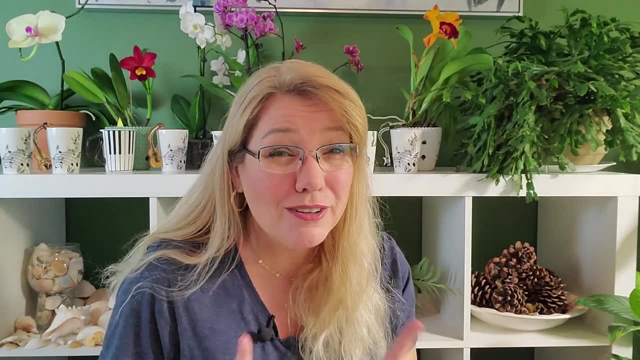 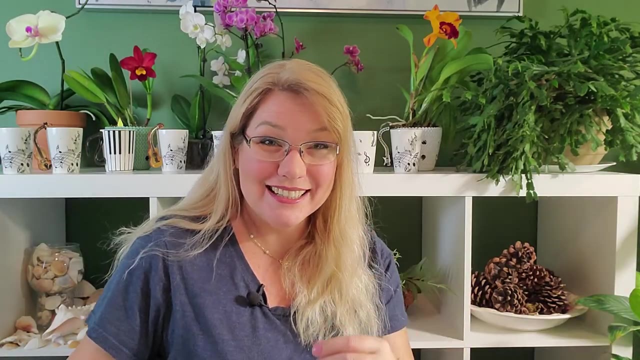 something on an impulse buy, which I usually don't do. I'm usually very calm and controlled and think about it and manage my budget- but this I could not pass up, even though I knew I was going to regret this later. So let me introduce you to my newest addition, a blue orchid. Now, why do I say? 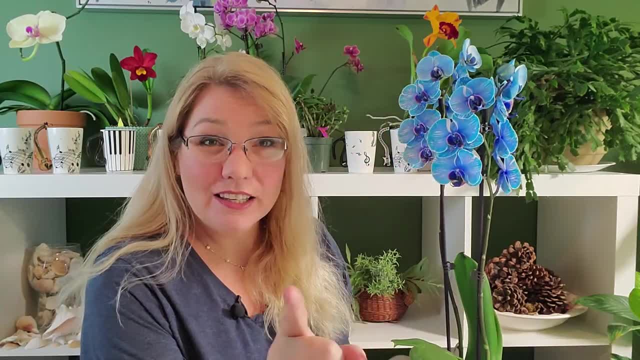 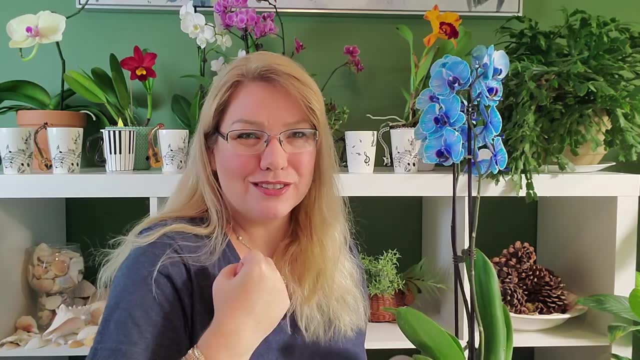 that I'm going to regret this later. Because, even though at first, look at those mesmerizing colors, this dark, deep, rich blue that just pulls you in and makes you want to just look at the orchid forever, I mean, look at that. 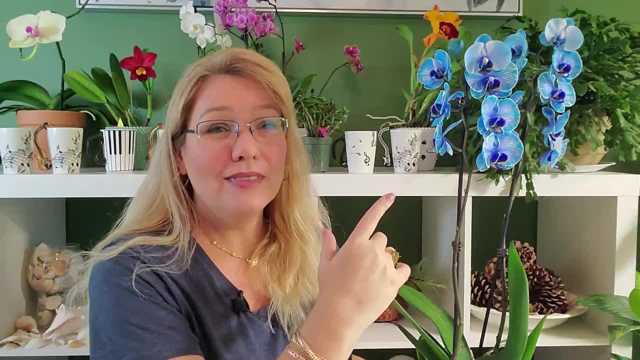 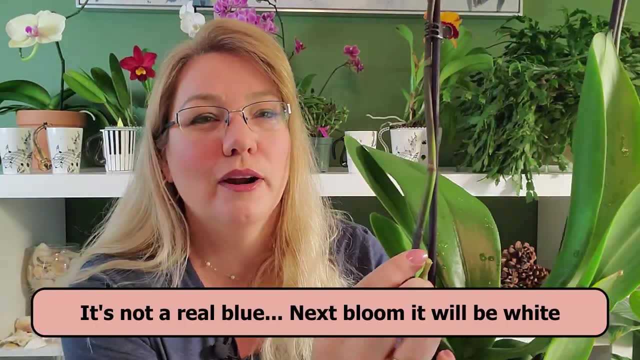 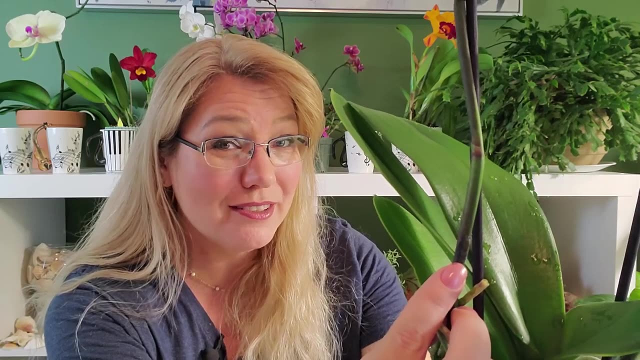 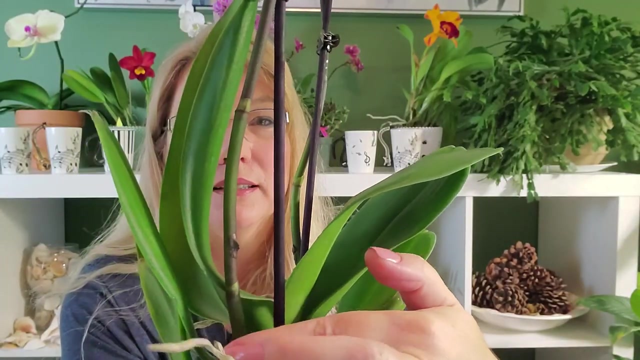 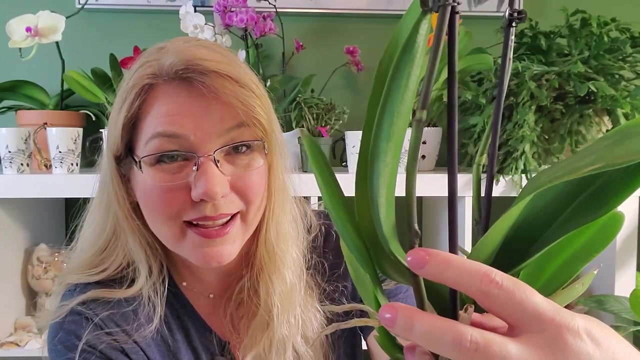 Isn't that just awesomely amazing? No, I am going to regret this, because right there is where they injected blue dye into a white Phalaenopsis orchid. Now here's this one, and here, let's get these really roots out of the way. Here is the second one. So on each flower spike, they injected blue dye. 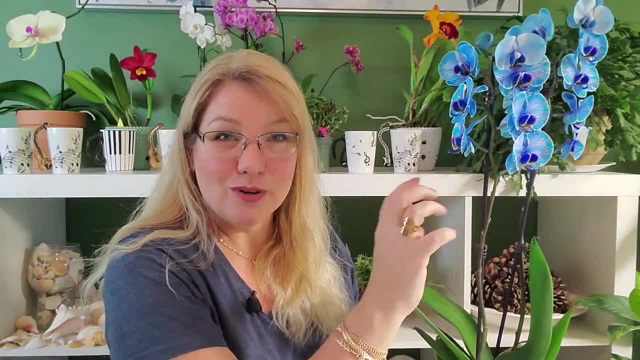 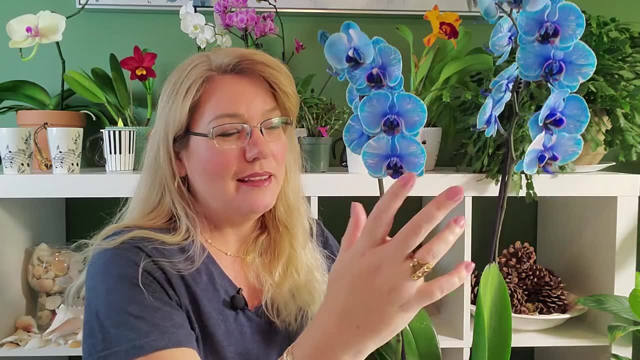 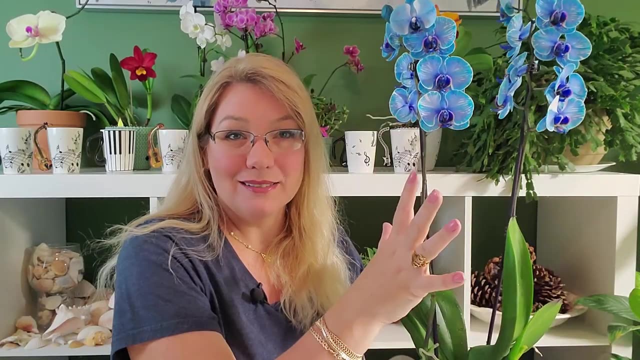 into this orchid. The older blossoms are going to be this dark, rich blue, while the younger ones are going to be a lighter blue color. Now, this will last because it was injected in the flower spike. this will last for one blossom only Next time. 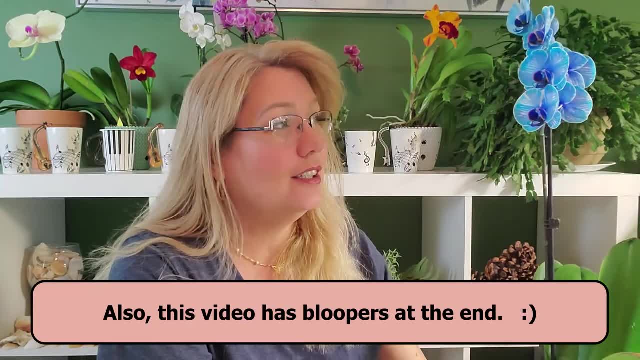 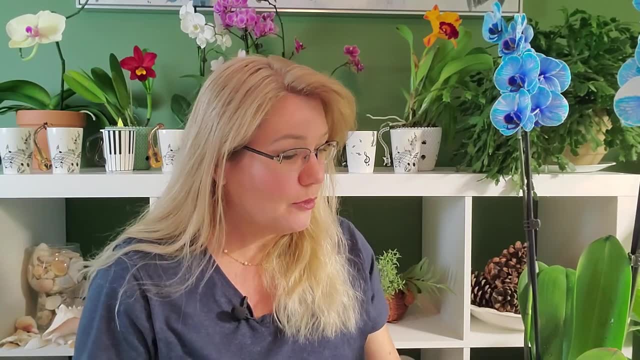 next year when this re-blossoms, it will last for one blossom only. Next time next year when this re-blossoms, or if it re-blossoms twice a year, it's going to blossom a white Phalaenopsis. So I'm going to regret it because, yes, I paid a heck. 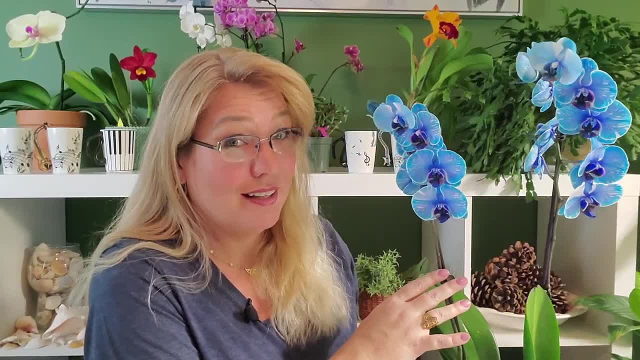 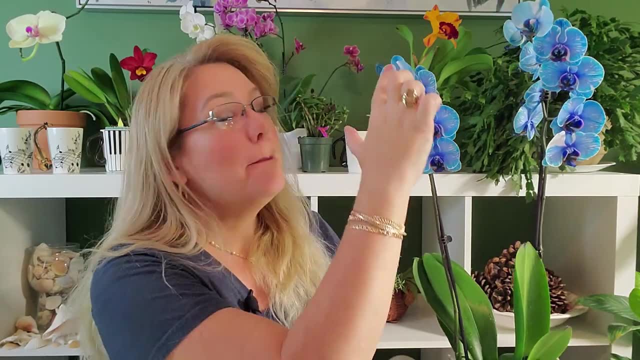 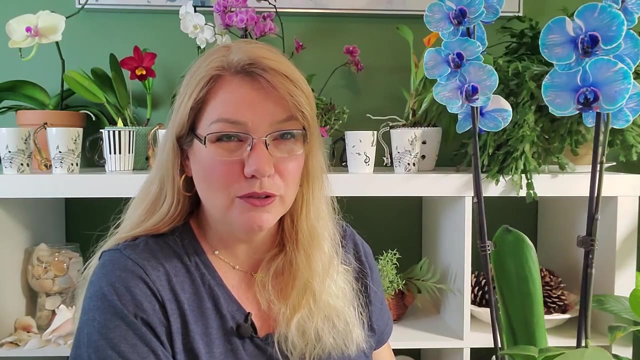 of a lot of money for this to be a white Phalaenopsis. nothing against white Phalaenopsis, I just think they're plain. My opinion only. But I had to have it. So the first step you get when you have this orchid, this beautiful blue orchid, is when you have this orchid, this beautiful blue. 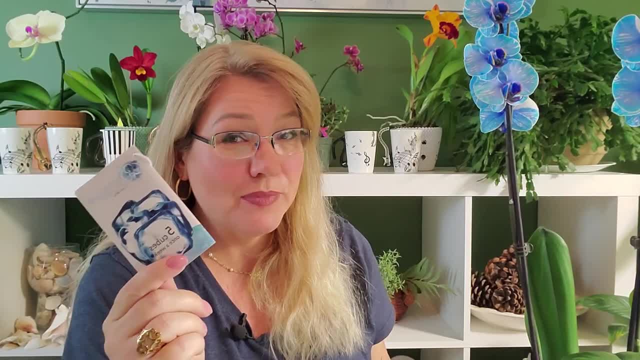 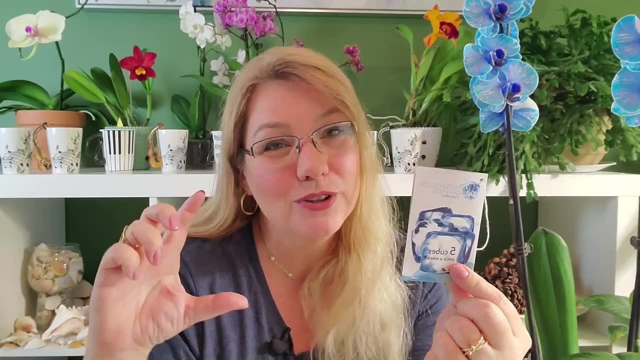 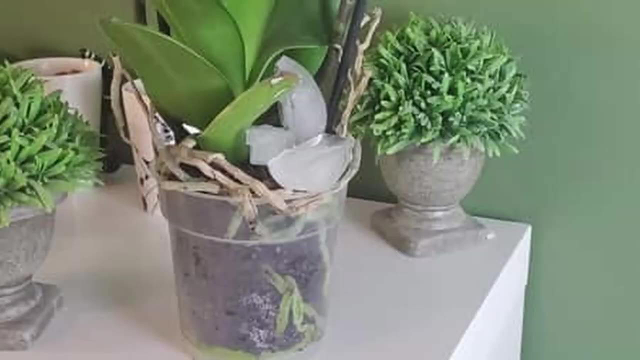 orchid. is you're going to read the instruction card Now? on the instruction card it will say, right on the cover: water with five ice cubes a week. Now, when you buy a mini Phalaenopsis, it says water with three ice cubes a week. This one says five. Well, it says five because look at, 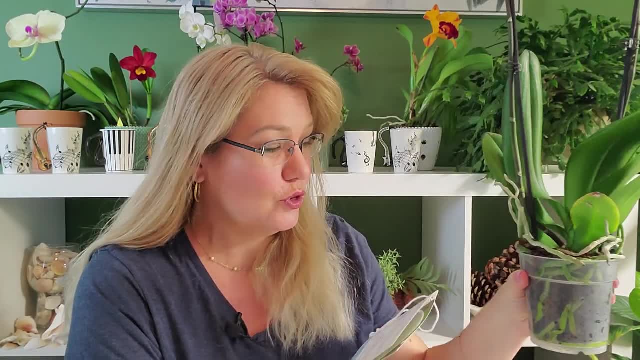 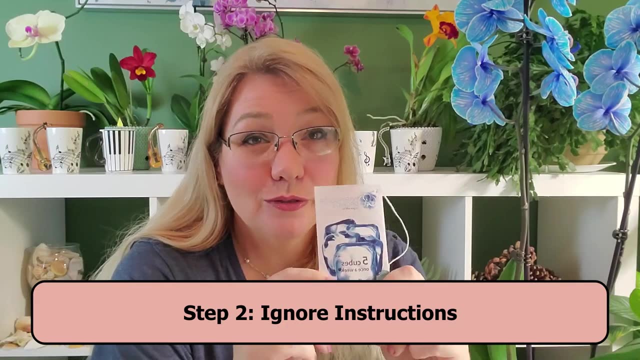 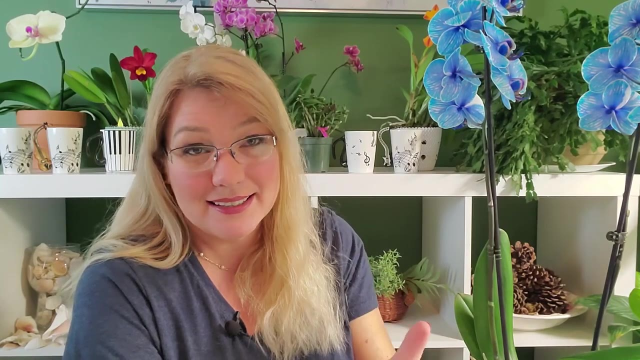 the size of that pot. It's amazingly huge. If you want your orchid to bloom next year and keep alive and keep healthy, well, first you're going to ignore this. Now you already know that this is going to re-bloom next year, or it could re-bloom in the next six months, but it will not be blue. 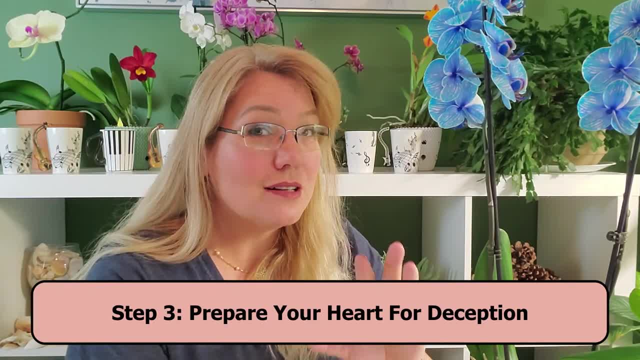 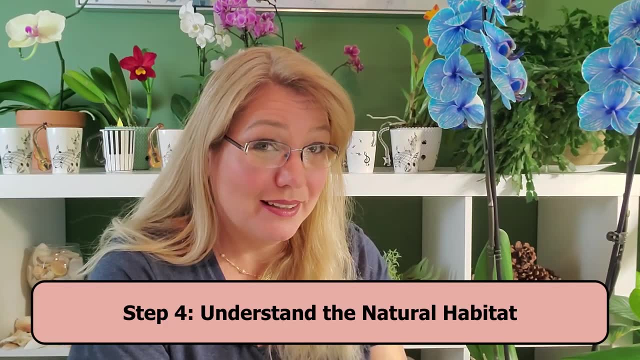 So you already know that Already. prepare your heart that you know, so you don't have a huge deception. Well, usually Phalaenopsis grow in a tropical climate. There is high humidity. They grow attached to trees, They grow attached to the barns. 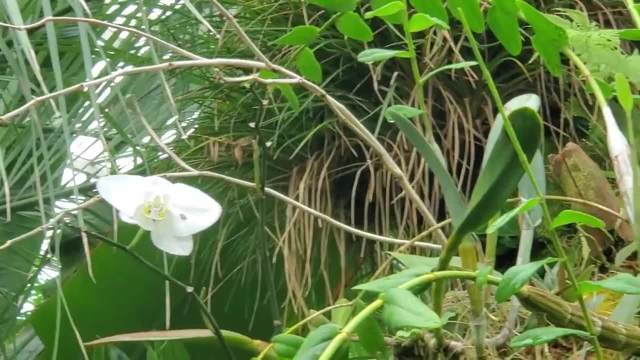 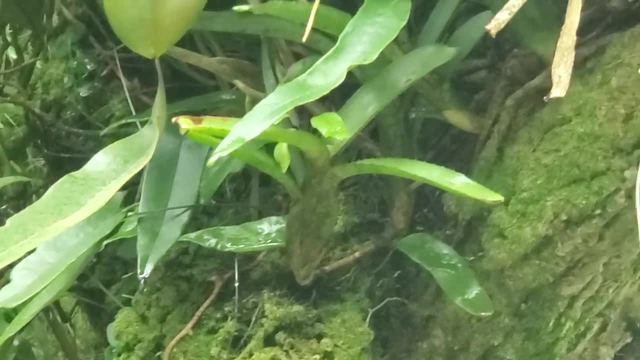 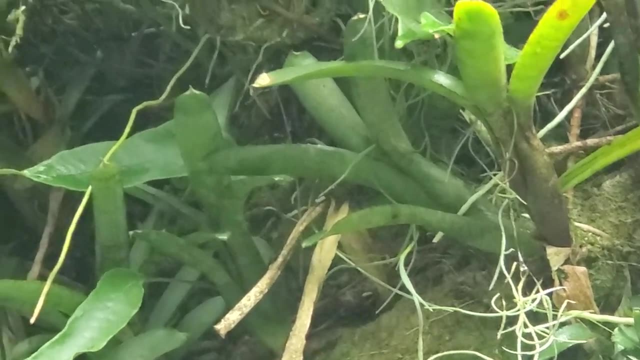 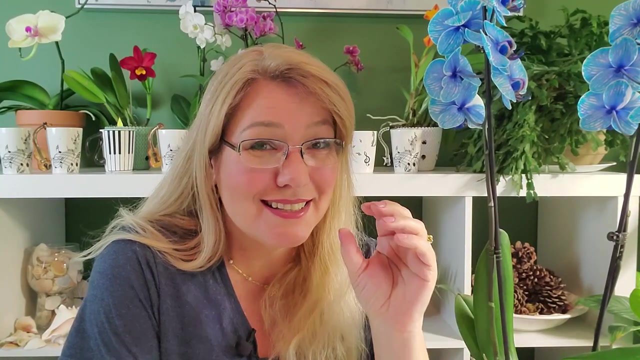 They're not going to be a parasite in the sense that they're not going to suck nutrients out of the bark. They're just going to hold on to that bark. That way they can be higher up on the tree to the sun, because in rainforests we usually have this idea that the soil on the rainforest is. 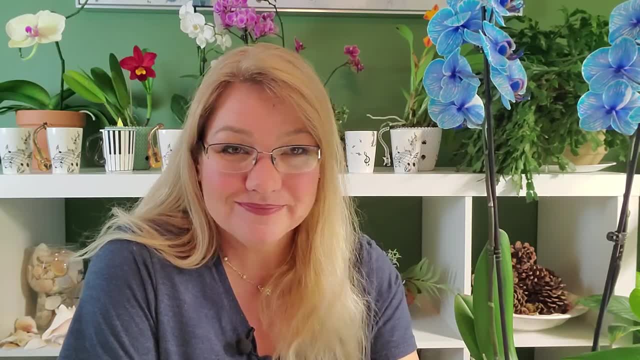 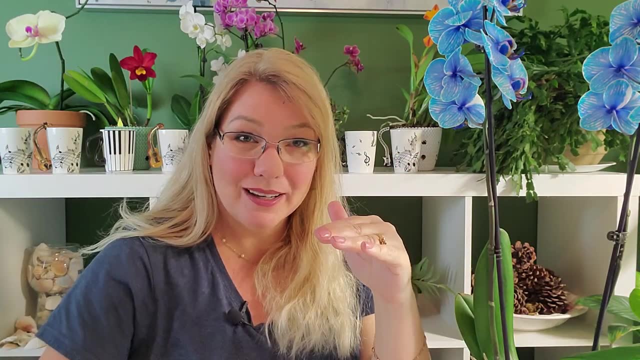 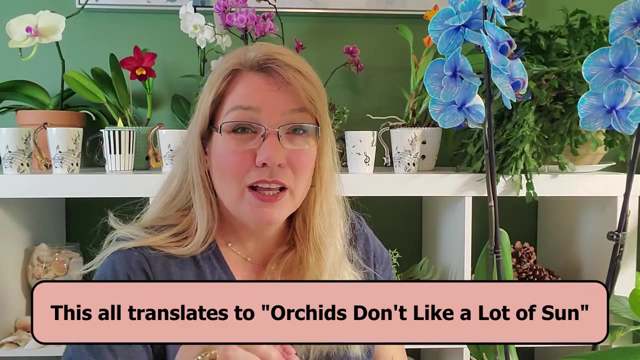 extremely rich in nutrients? It's not. It's really not. It's so thick on the canopy of leaves that the sun doesn't penetrate them all the way down to the ground. So the sunlight that reaches the soil is only about 20 percent. So when the orchid attaches, 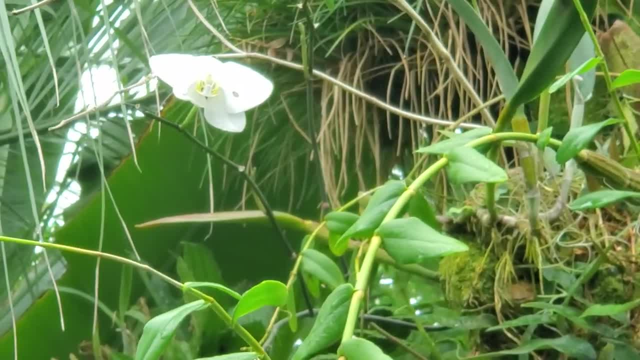 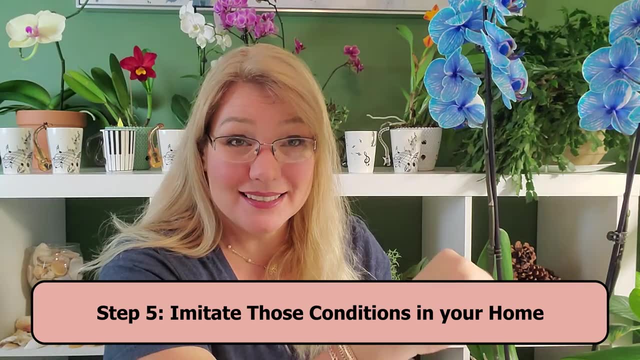 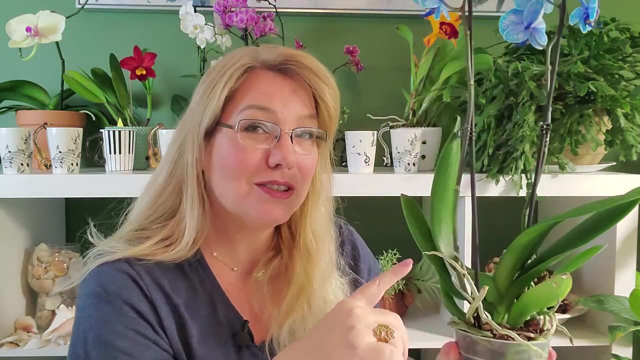 itself higher up on the tree. it's going to receive that adequate light. They like bright light but they don't like direct sun, So you won't. you want to keep this orchid on a window seal that has like a sheer curtain that's going to get sun in the morning hours only, and probably only around the. 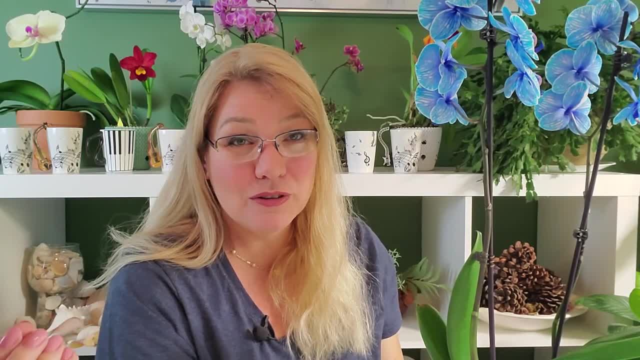 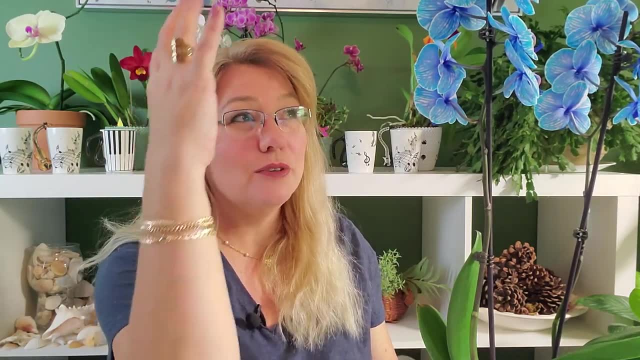 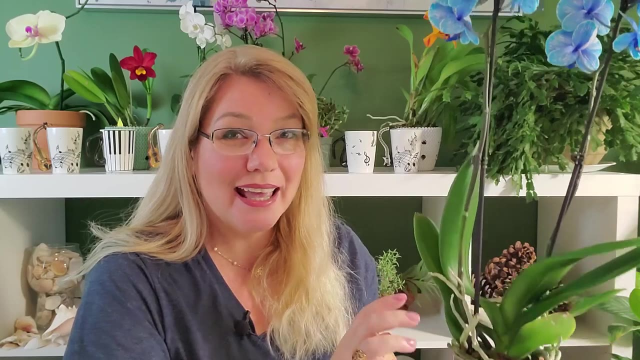 maximum two hours. So if you have an east facing window where sun can come up early in the morning and just shine on those leaves, you don't want to put the sun where it's getting on the blossoms because that's going to make them fade sooner. You're going to want the sun on the leaves and 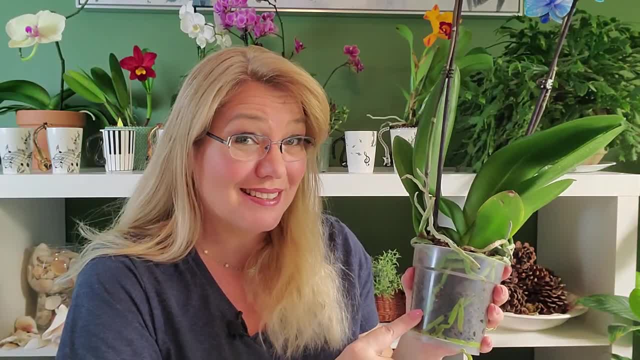 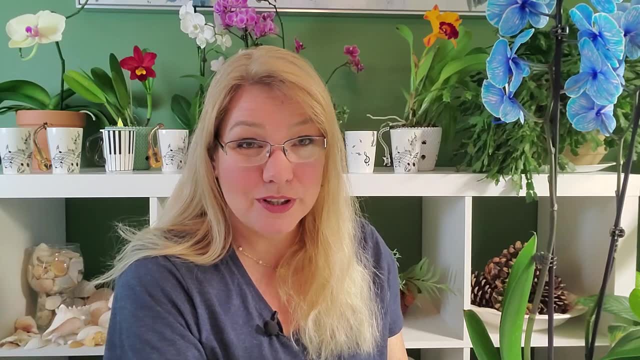 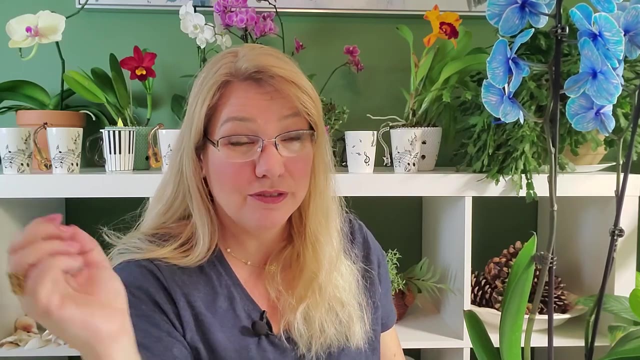 on the roots, because orchid roots photosynthesize. They're different than household plant roots. So you're going to keep this orchid in a east facing window. You are going to want to keep it away from direct hot sunlight- If your sun, that's. 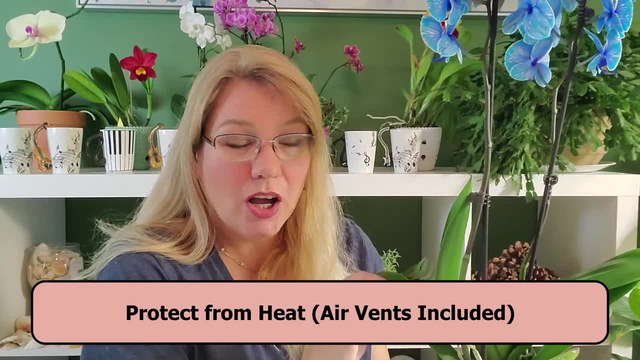 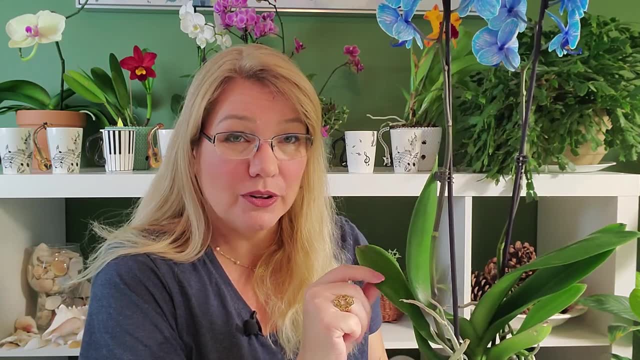 coming in on the east facing window is extremely hot and you touch this leaf and it is just hot to the touch. it's getting way too much sun and it's going to sunburn. Orchid leaves sunburn because of heat and because of direct light. 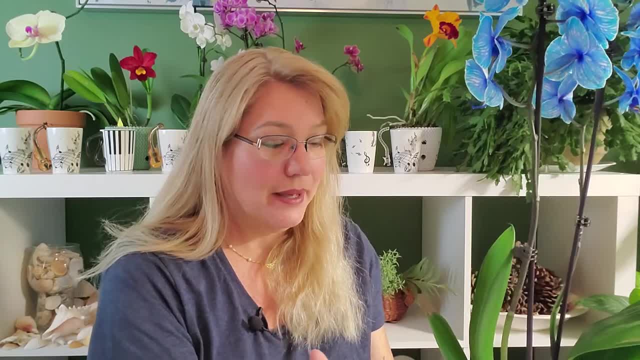 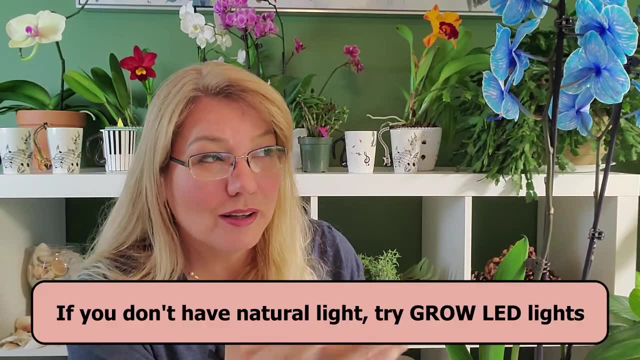 So you want a bright space. You want a space that sun will get to it, but not direct sun. If you don't have that- like I don't- When I bought my house I had I don't. I mean, I love the neighborhood, but I 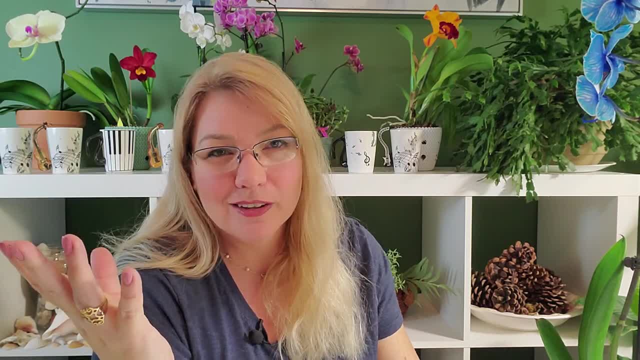 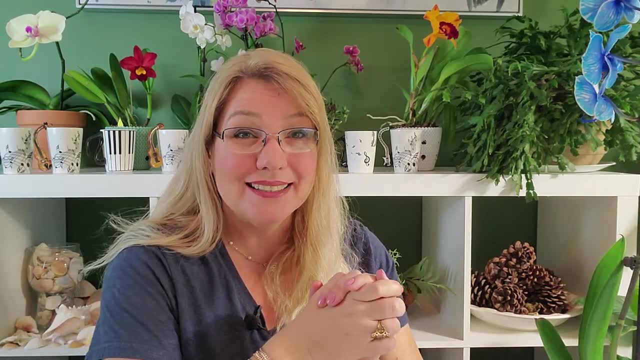 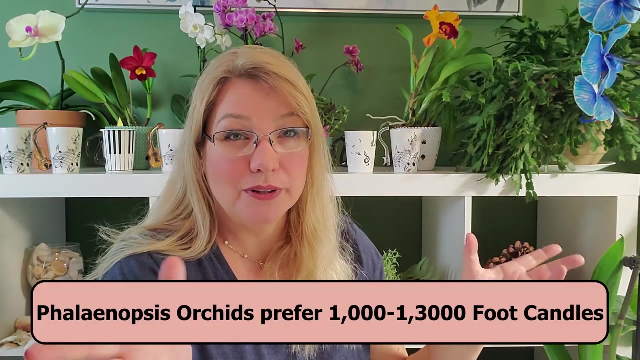 really didn't think about orchid lighting. You don't think about that stuff when you buy a house. So after I moved in I was like, yes, where am I going to put all my plants? Nowhere, I have a grow light. They're not that expensive and they do great for my orchids, So I have to grow all mine totally. 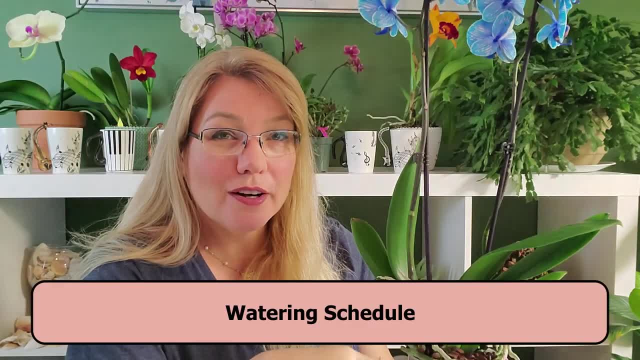 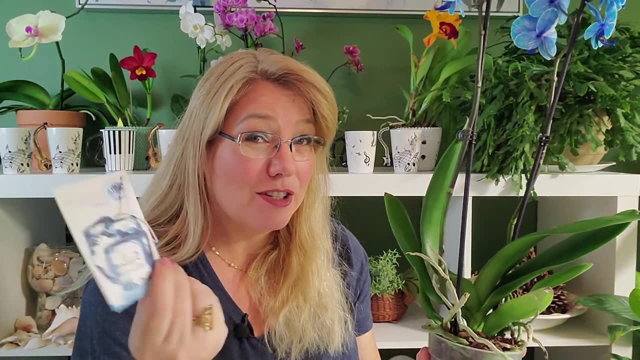 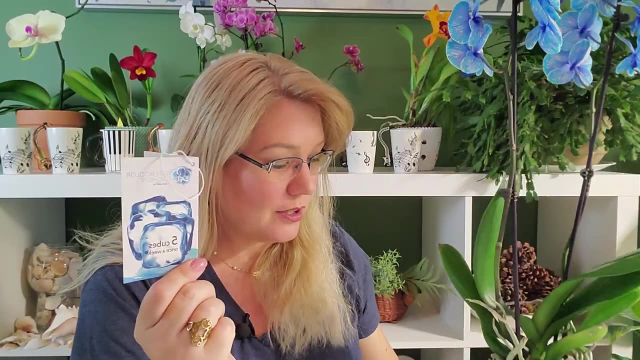 indoors, That works too. Watering. Your biggest problem is going to be because on the card that it comes with the information card, there's a huge picture right here of ice cubes. Now think about how this orchid was grown in nature. It's in a tropical climate. It's never seen a day of cold. 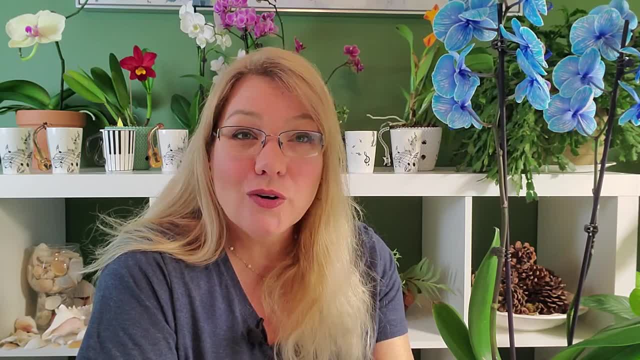 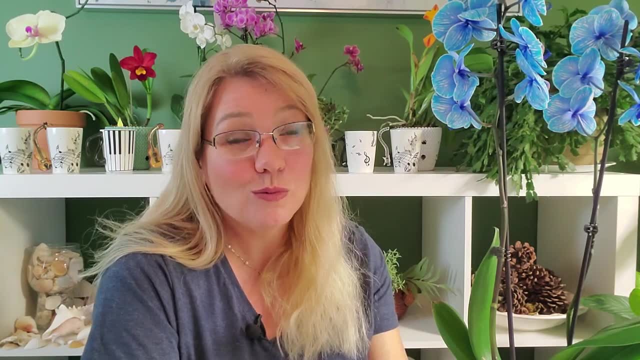 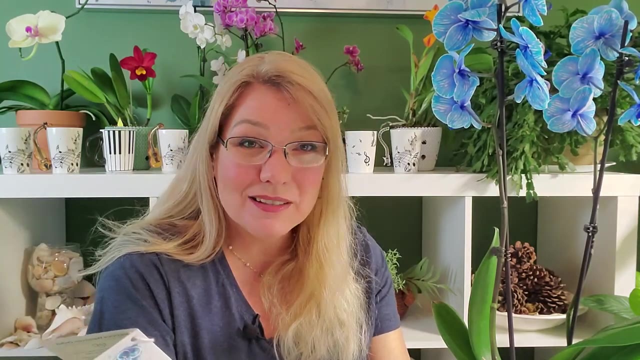 water. It's never seen a day of cold water. It's never seen a day of cold water. It's never seen a weather in its life. Orchids grow on every single continent, except where there are glaciers. They don't like cold water. Now, will this method work? Yes, obviously it will work. Is it the best? 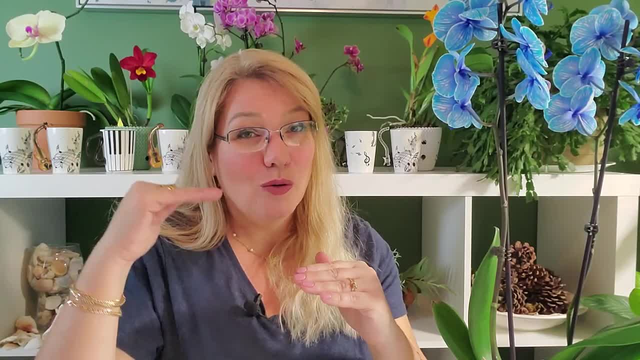 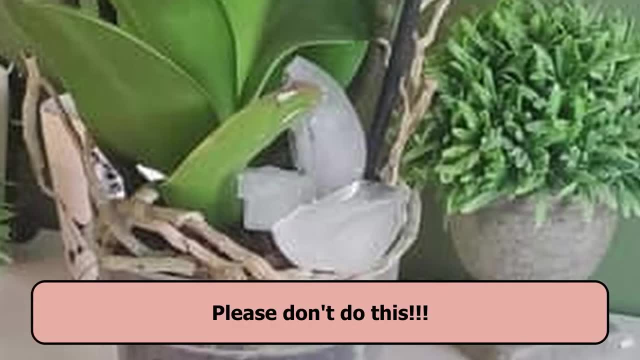 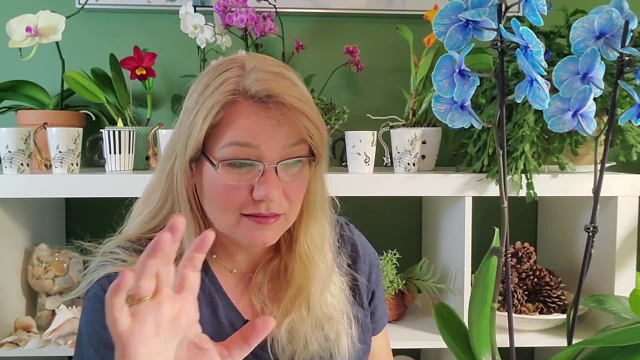 method. Now see, there's a difference between watering with ice cubes and your orchid living and giving the best orchid care that you can to make this blue orchid really thrive. So you're not going to use ice cubes, You're just not. First, when you put ice cubes on there, it says: 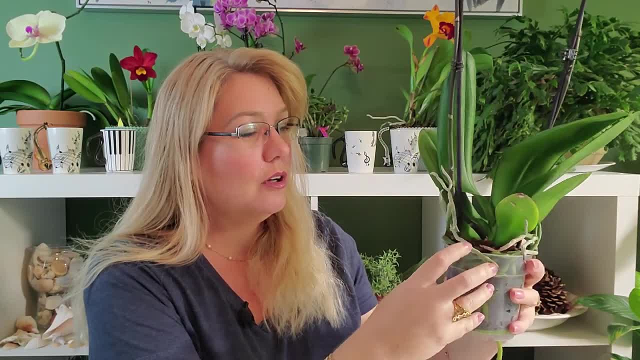 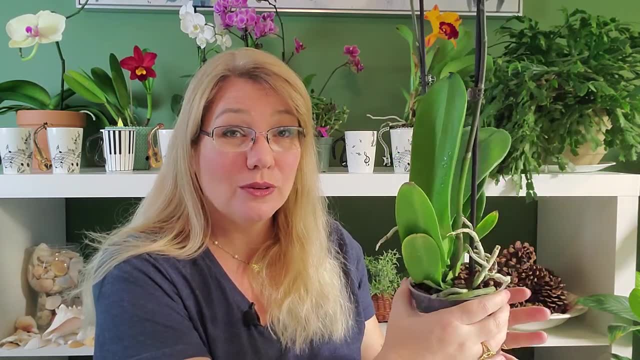 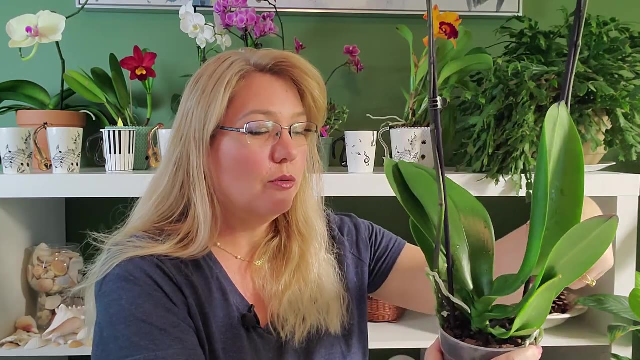 water with five ice cubes. Well, if you water with five ice cubes, it's only going to hydrate the place where the ice cube sits. You're going to want to take this orchid to the sink, or you're going to want to water it inside a bin, Put it in a plastic tub and pour water around the whole pot. 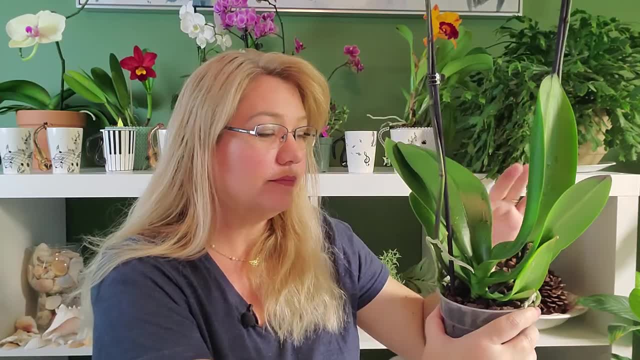 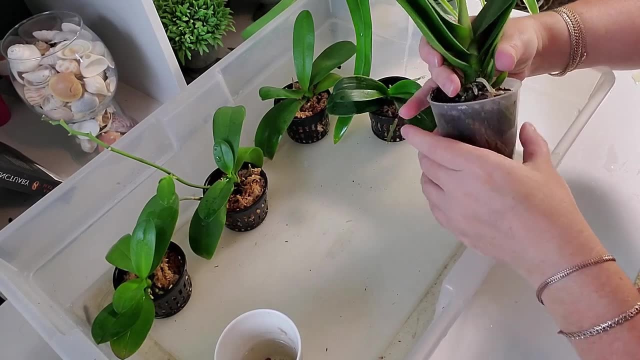 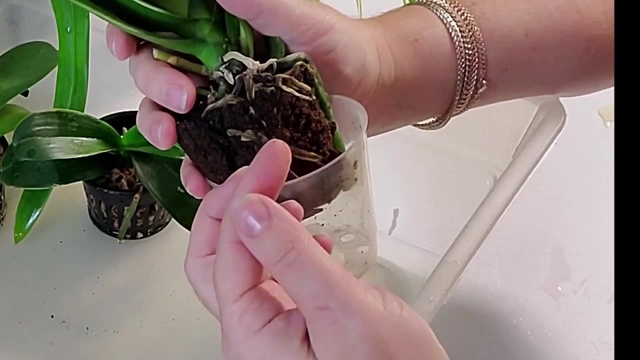 except for the middle, The crown. If you have a, just add ice orchid, their potting media is going to be a little bit different And let's see if I can. yeah, see, it's like this brownie stuff cake like peat moss is. 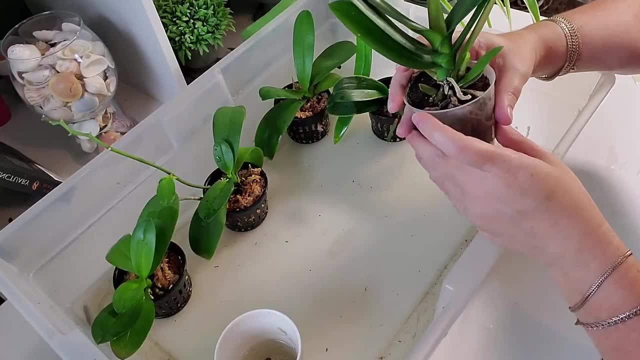 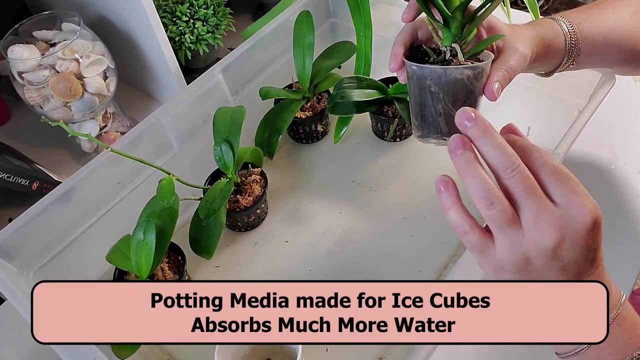 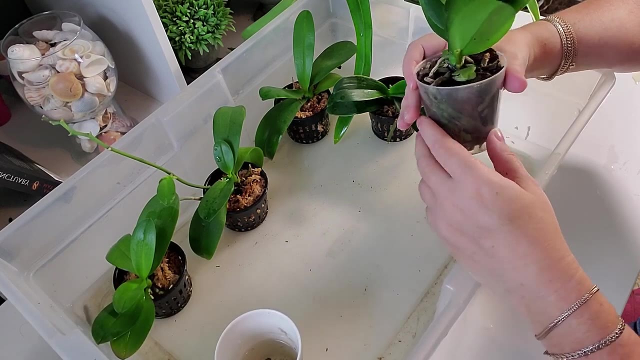 actually what it is- mixed with some other things, And this medium will retain much more water than any of the others In sphagnum, moss, orchid, bark, perlite, charcoal. this is actually the worst media to be watering in because it absorbs so much. 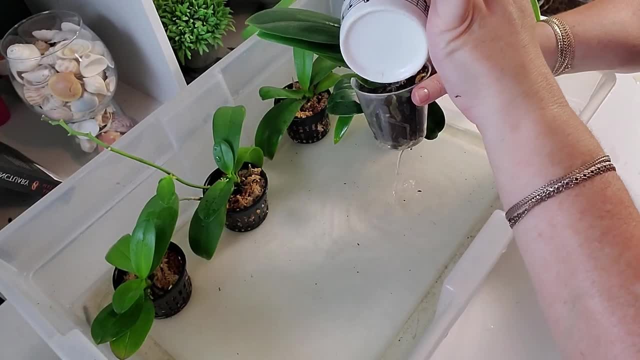 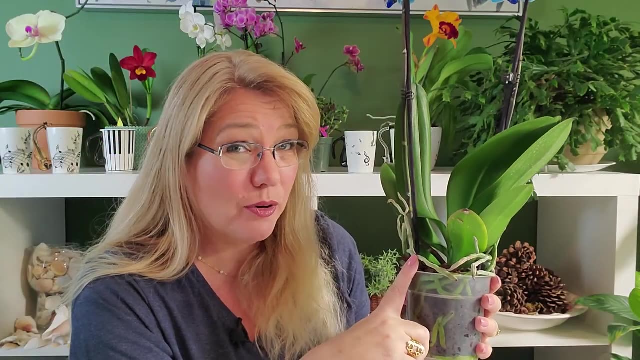 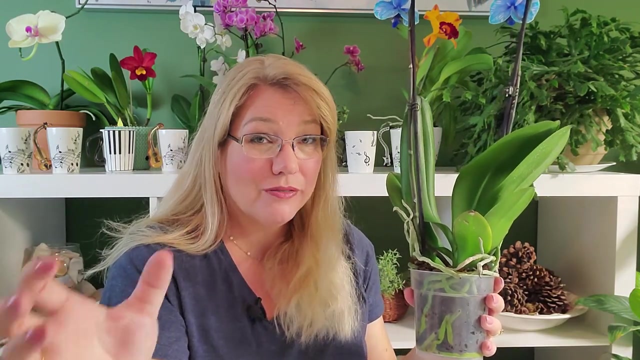 if you get your water and pour it on here like this, it will absorb almost all that water. if you put tap water on here, it comes with a whole bunch of minerals that the orchid doesn't like, especially chlorine. so get your tap water if that's the only water you have. 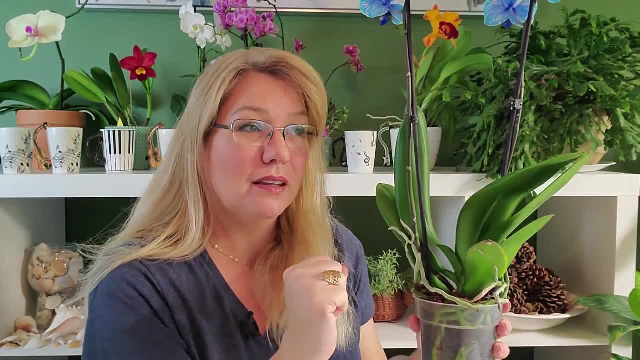 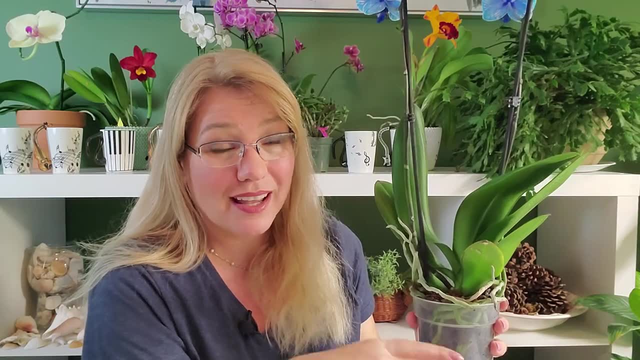 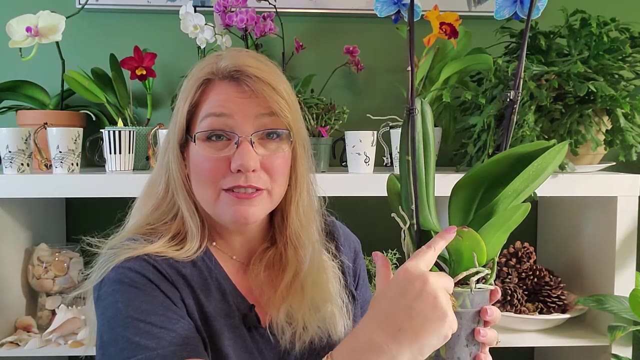 get your tap water, leave it out of the. leave it like in a bucket overnight. that chlorine will evaporate and the other minerals stay. but the chlorine will evaporate, so it at least it's not that harmful if you start to see your leaves turning yellow like a 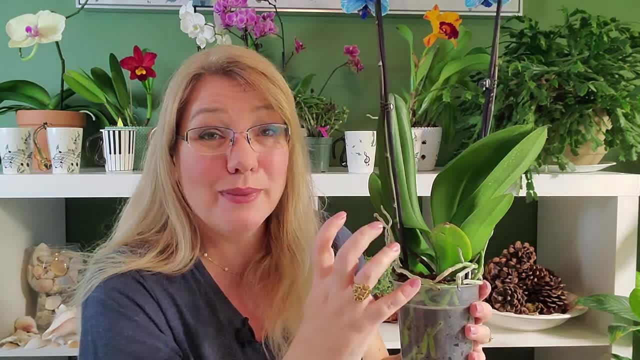 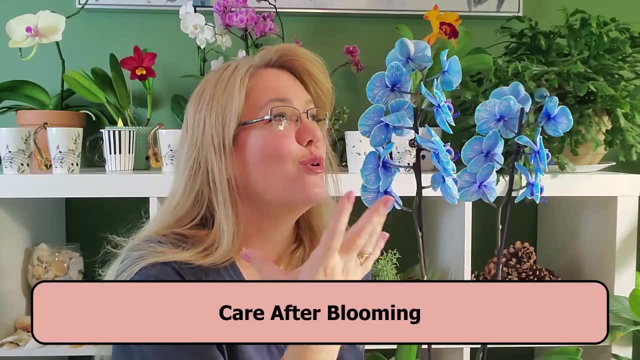 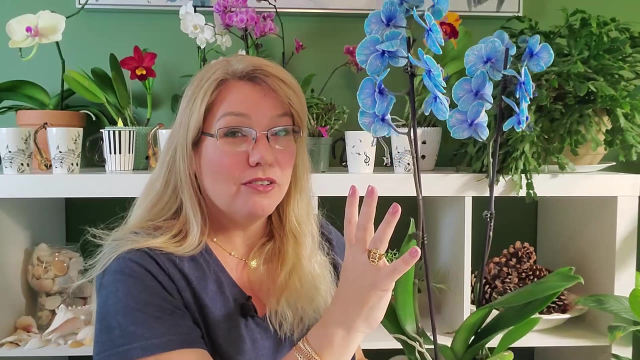 deep yellow. that's probably because you've got too many chemicals in your water. after the blooms fall off, because you're going to want to, i mean, just enjoy it, these amazing blooms, for the most amount of time that you have. so after they fall off, repot you're. going to want orchid, bark and sphagnum, moss, perlite and charcoal or activated char, activated carbon. you're going to want those four, depending on your climate. you are going to need a humidifier because in their natural habitat, orchids do stay in a relative humidity of higher than 40 percent, and 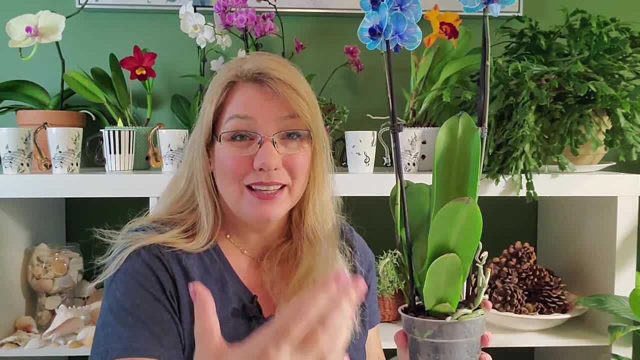 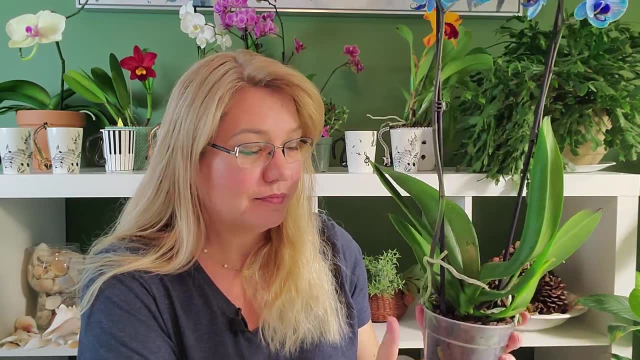 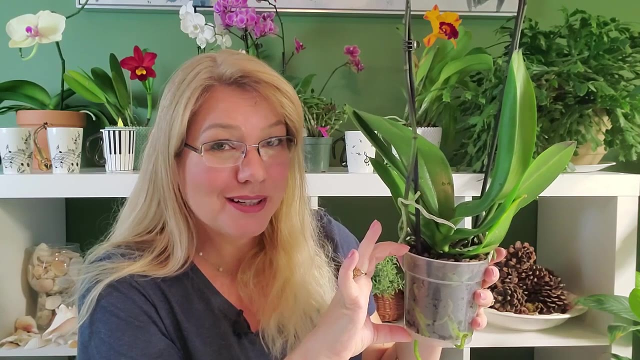 our homes with the, with the heating system and the air conditioner, are around 27 to 33 percent. if you don't want to invest in a humidifier, you can use a humidity tray, but in this case, since the orchid pot is so big, the humidity tray isn't going to add that much difference. 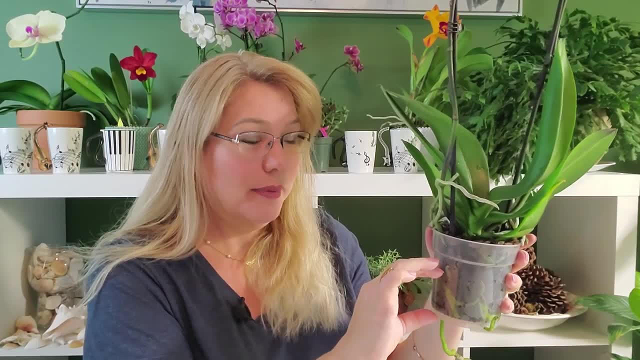 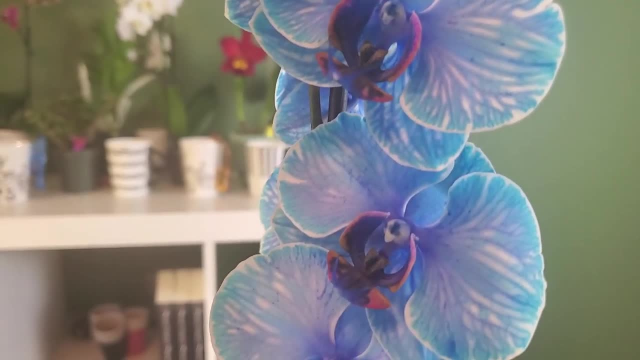 you're going to want to use a humidifier, because in their natural habitat orchids do stay in a because humidity trays are only going to make a difference about two inches from the top of the tray. if you had a mini fowl, the humidity tray would make a lot of difference. so you have your. 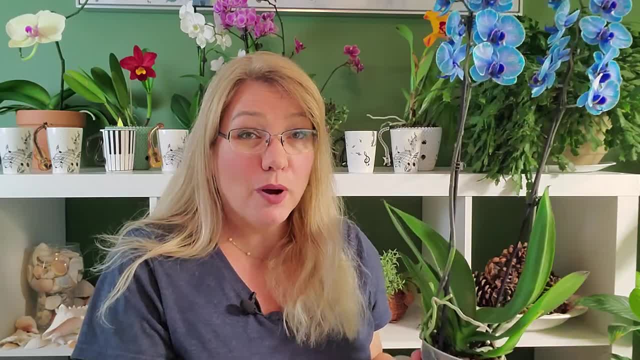 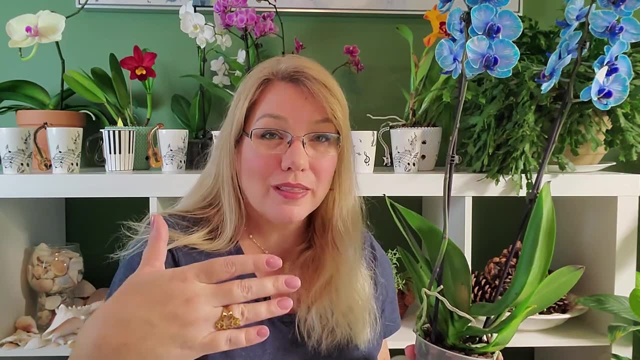 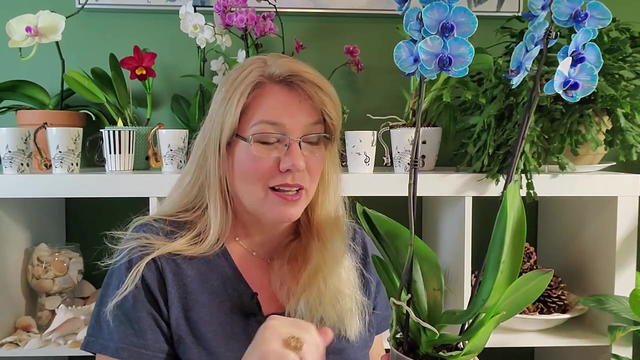 watering. you have your lighting, you have your repotting every two years and you need a fertilizer every fourth time you fertilize you water, you'll need to add a tiny, tiny, tiny bit of orchid fertilizer. this will keep the plant healthy and strong. if you don't want to use store-bought, 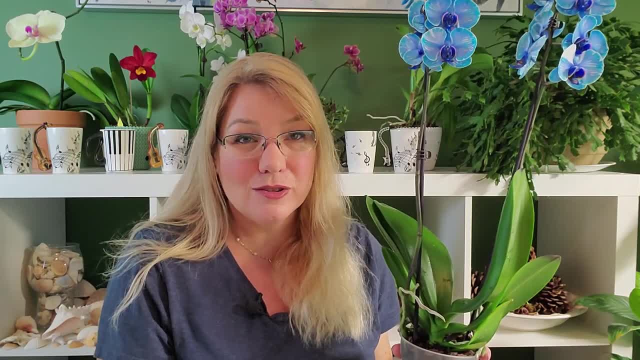 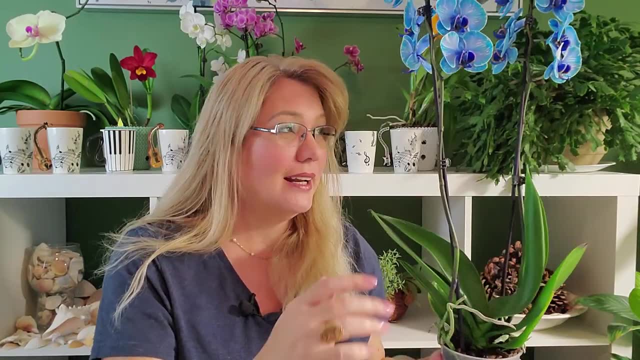 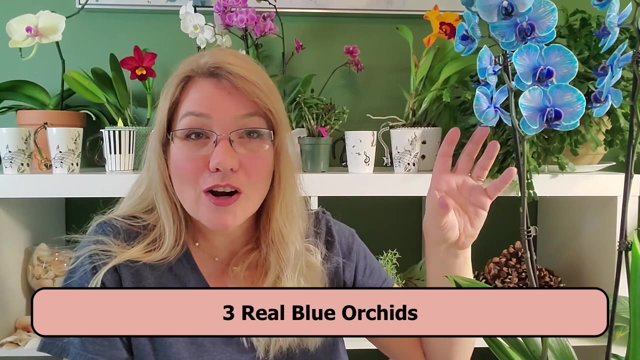 fertilizers. there are a whole bunch of other methods you can use. but take it slow, you know. first get your watering right, first get your lighting right, the humidity right, then you can enjoy your orchid for a long time. why is it so hard to find blue orchids or blue flowers in nature? 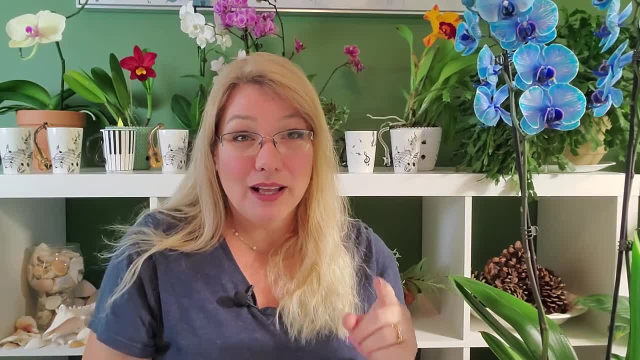 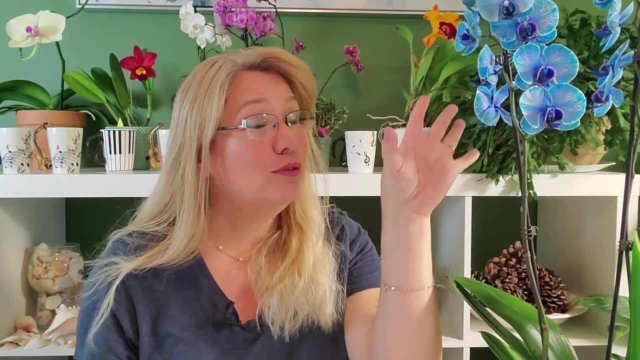 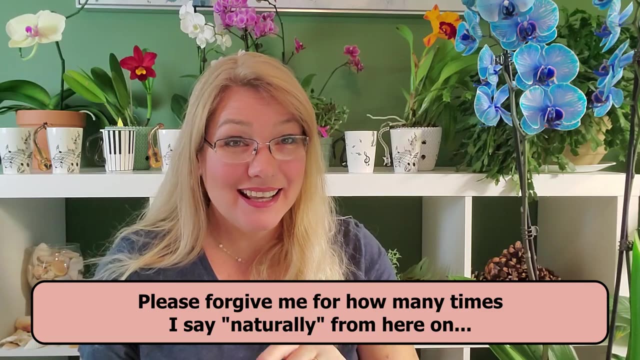 less than 10 percent of the orchids that you can find in nature are blue orchids. so if you have a 10 percent of all flowers have a blue pigment in them in nature. that is why it is so hard to find these blue flowers naturally. but there are three naturally blue orchids in nature: felimitra crinite. 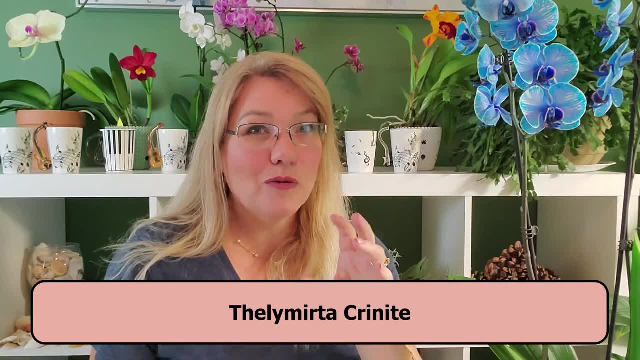 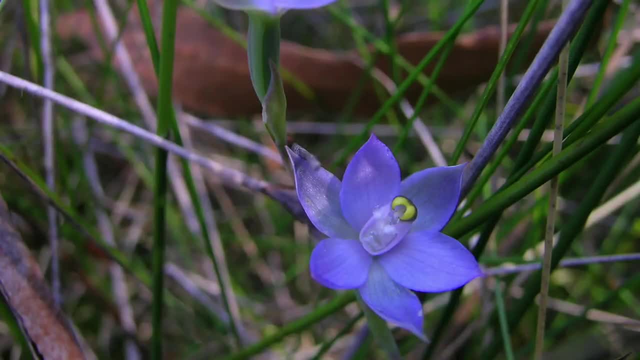 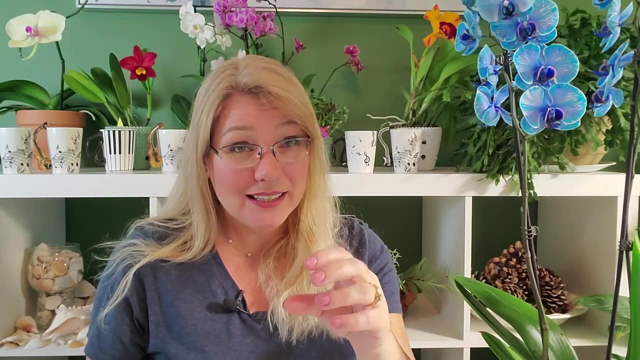 is a naturally blue orchid with no purple, no lavender tones to it. it's the darkest blue that will naturally cause in nature. sometimes you can go to an orchid store online and say, hey, we've got this indigo orchid that has been manipulated and it is true blue, but it's not. 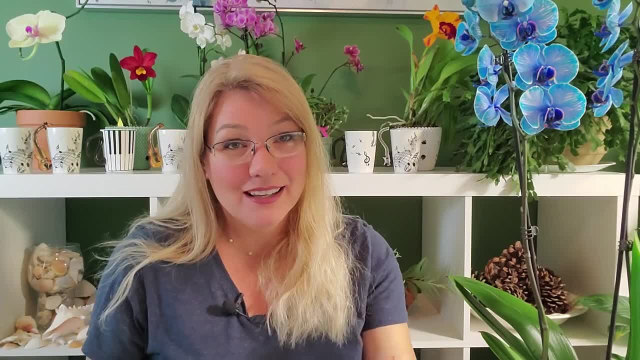 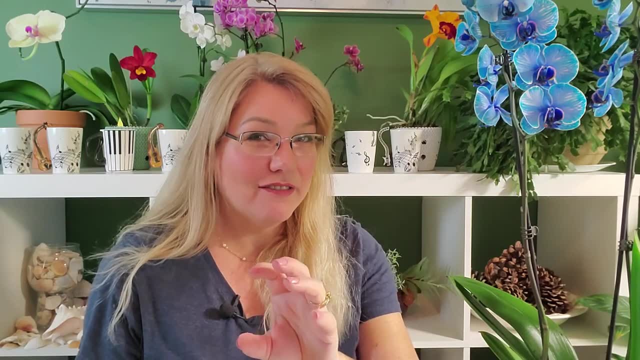 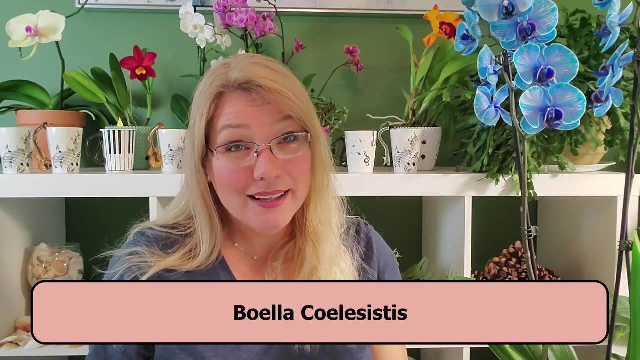 one that nature came up with by itself. it's one that man interfered with. felimitra crinite grows in new zealand and australia and they do not have that lavender or purple tones to them. they are a natural indigo color. the second blue orchid is the boella coelestes. now that is grown in the 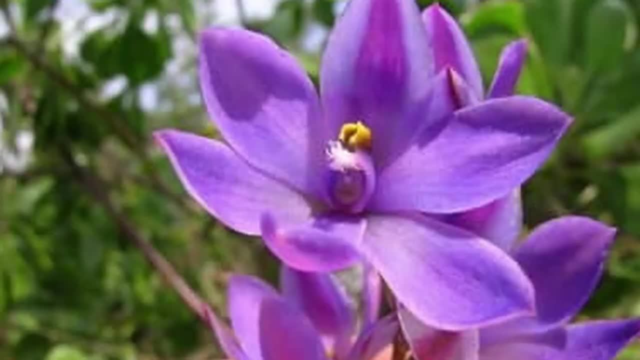 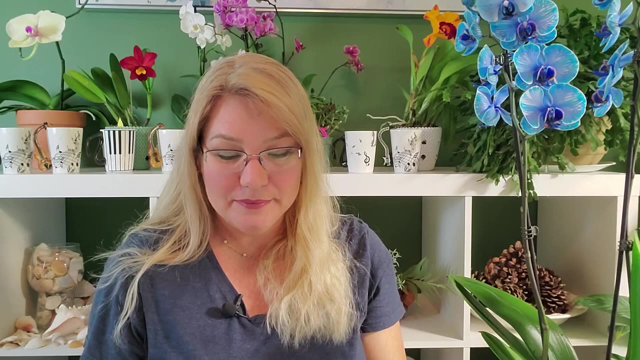 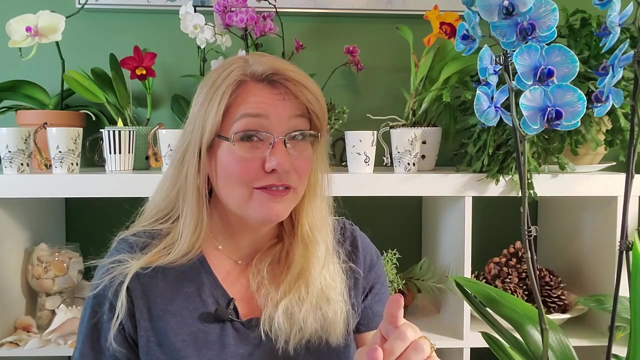 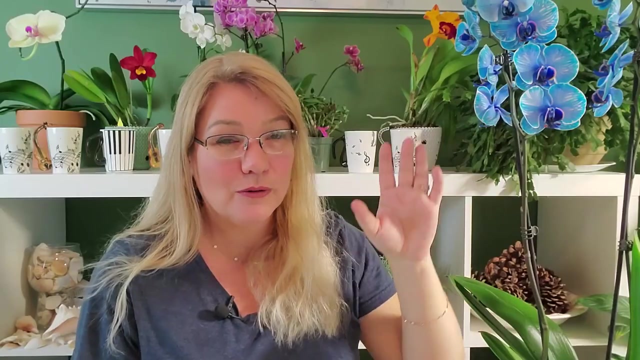 southern andes region and it is extremely hard to grow. you have to know what you're doing to care for one of these orchids. the third naturally grown orchid that is blue is the blue vanda. now you can find these online to buy and sell. they are a little more complicated than your phalaenopsis orchids. they